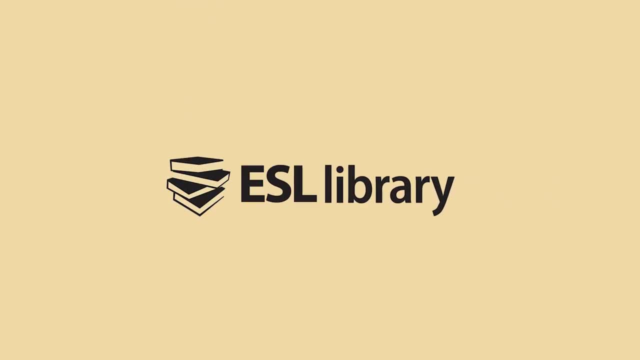 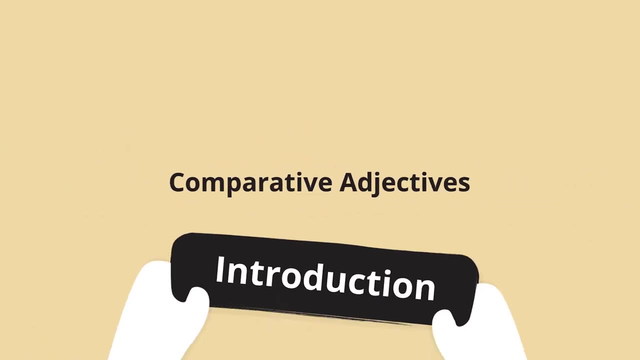 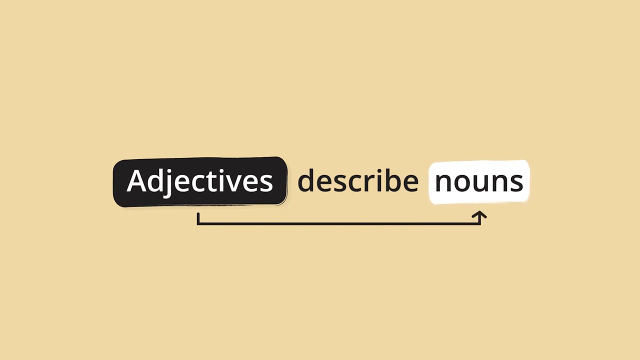 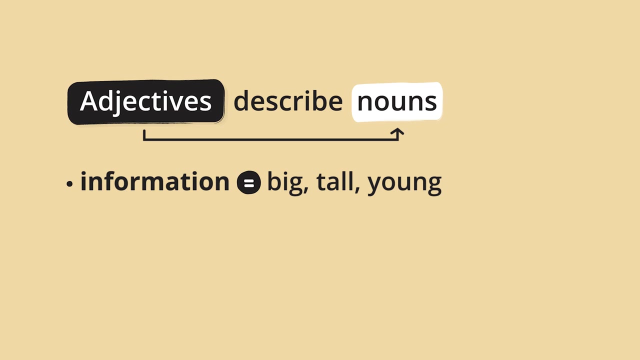 What are adjectives? Adjectives are words that describe nouns. Adjectives can give us information such as the size or age of a noun. Adjectives can also tell us someone's opinion about a noun or describe how someone is feeling. We use comparative adjectives to compare two people. 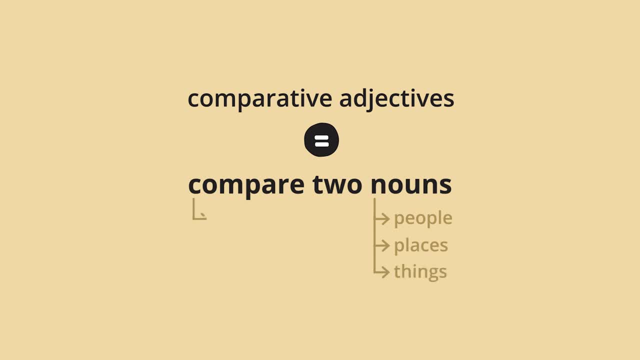 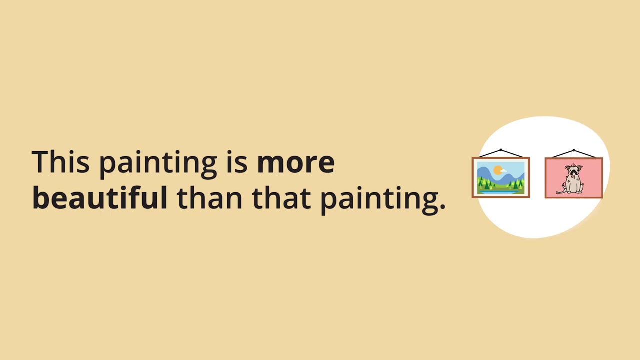 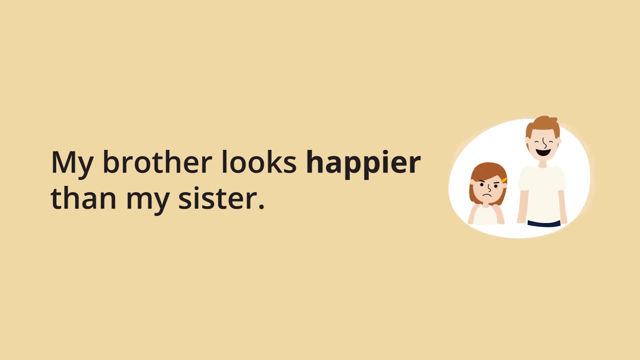 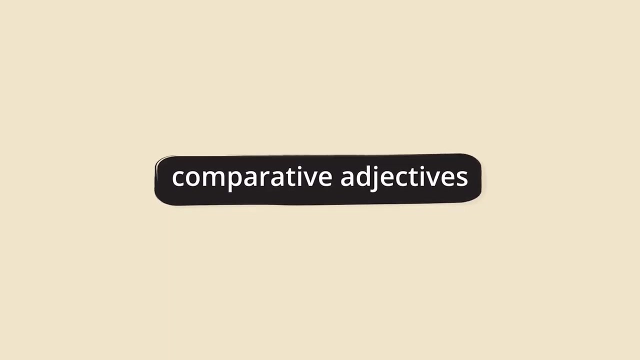 places or things. Comparative adjectives tell us how one noun is different from the other. For example, she is taller than him. This painting is more beautiful than that painting. My brother looks happier than my sister. How are comparative adjectives formed in English? It depends on how many syllables the adjective. 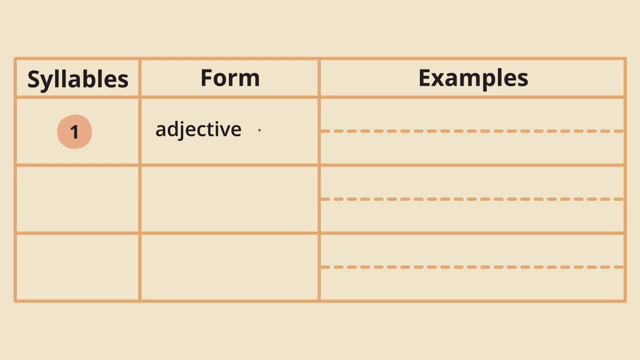 has. For one-syllable adjectives, we add er to the adjective. For example, short becomes shorter. If the adjective ends in a consonant-vowel-consonant pattern, we double the final consonant before adding er. For example, big becomes bigger. 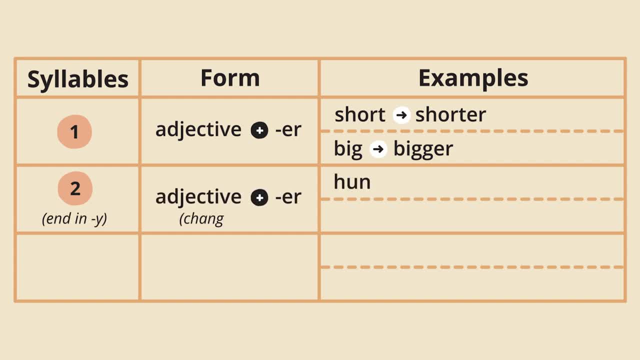 For two-syllable adjectives that end in y, we change y to i and add er. For example, hungry becomes hungrier and noisy becomes noisier. For adjectives that are two syllables or more, we use the word more before the adjective. 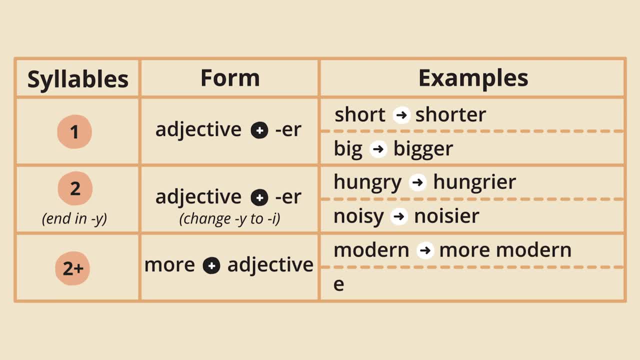 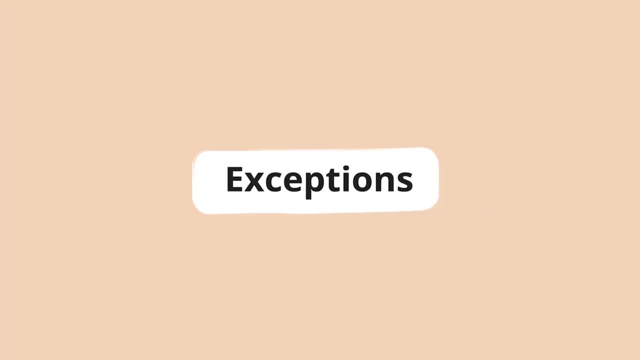 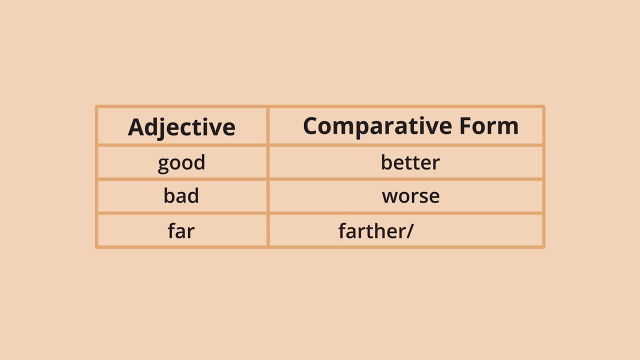 For example, modern becomes more modern and expensive becomes more expensive. Some comparative adjectives in English don't follow the usual rules. For example, the adjective good becomes better in the comparative form bad becomes worse and far becomes farther or further, The most common sentence pattern for comparative